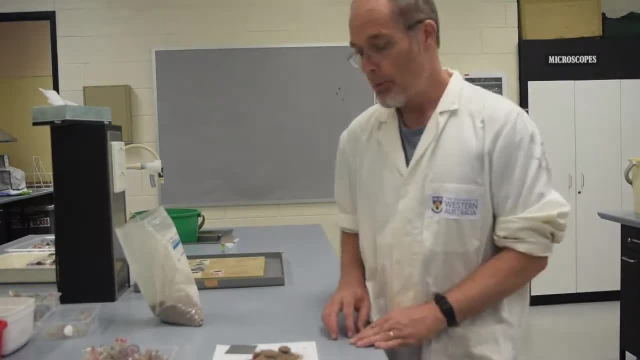 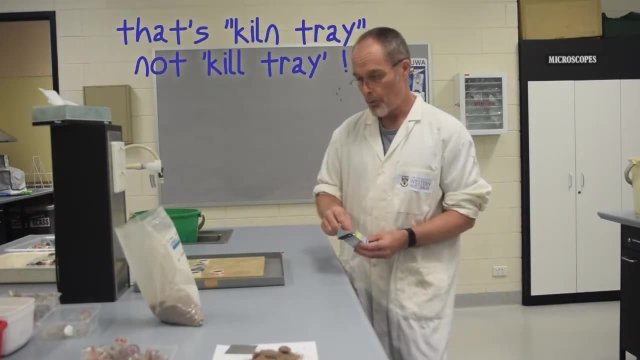 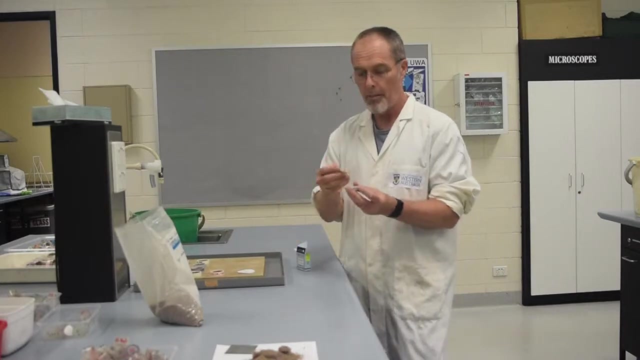 small samples to saturation. so for each sample we use a kiln tray, which is a porous ceramic tray sitting in deionized water, and we place a filter paper on there with a retaining ring which needs to be labeled carefully, and you'll need to read the lab manual to know how to label the retaining ring. so 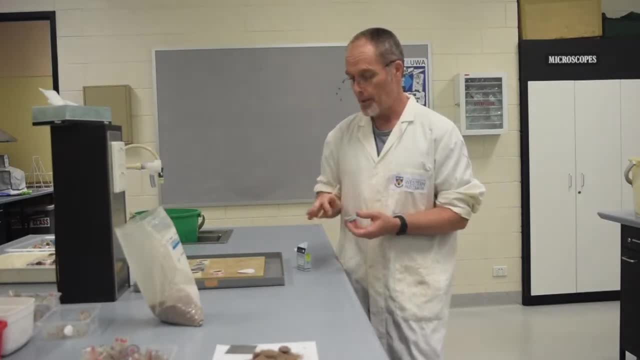 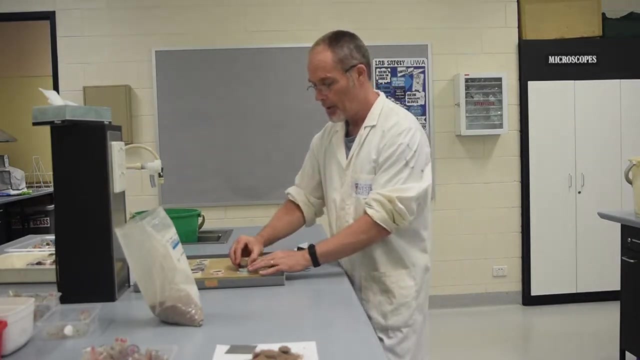 at least your name- and the pressure that this is going to be equilibrated at to modify the water content. so once we've got a filter paper there and a label retaining ring, we will just take one of these weighed soil samples and empty it gently into there. now what will happen is that the capillary action of the 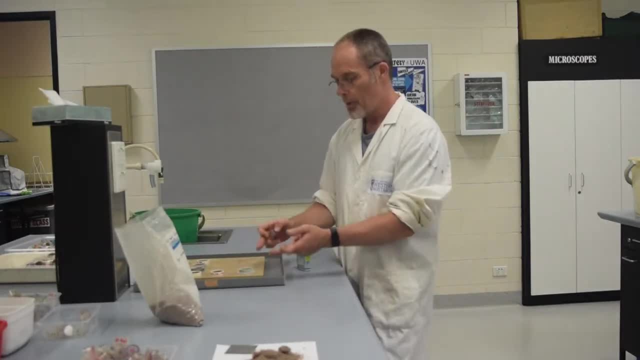 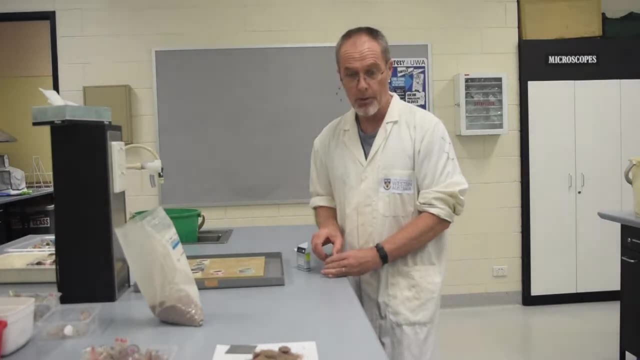 small pores in the kiln tray will draw up water so that this will the soil sample will become saturated. it will take a little while, but don't worry, there are things to do while you wait. for example, you need to measure gravimetrically the starting water content of your soil. it won't be zero. 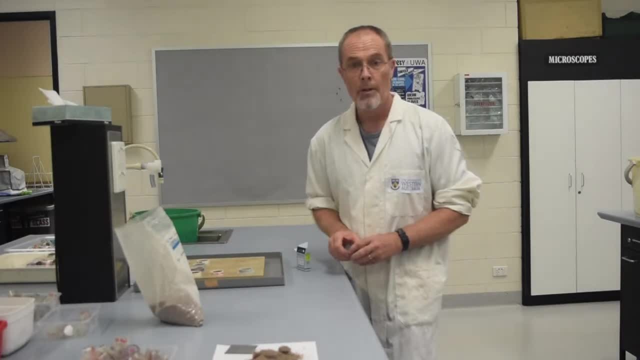 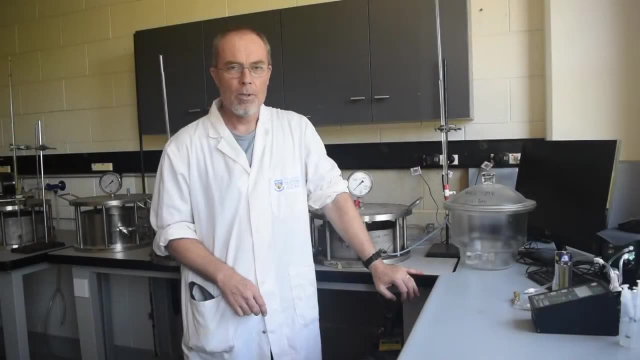 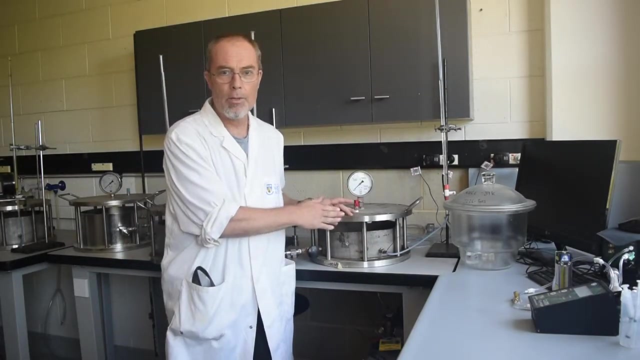 and you need to account for that in your calculations. all right, we need to stop there. now We apply the pressure to the soil samples in these very thick walled steel vessels here, so we can apply pressure in here up to about 1500 kilopascals above. 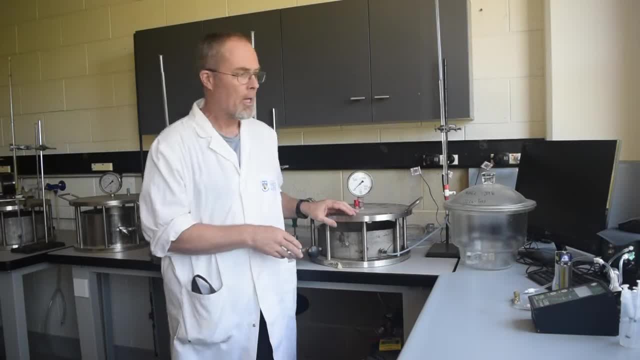 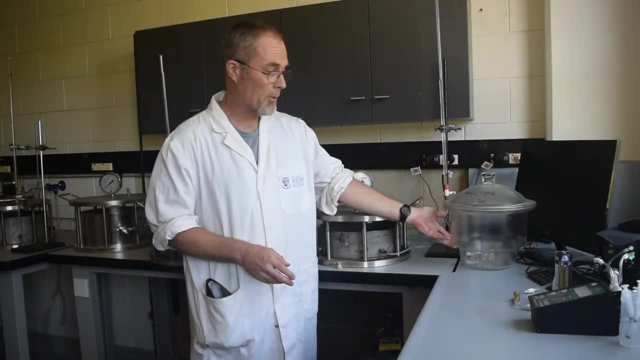 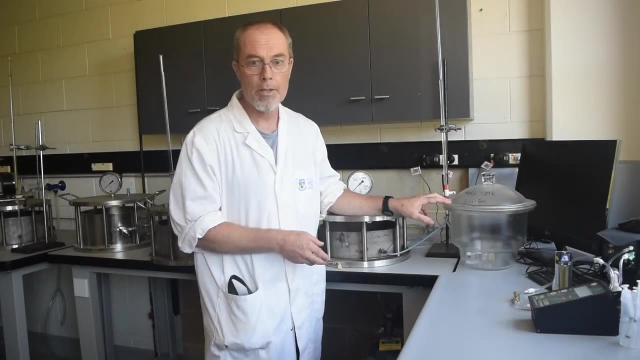 that we have to cheat a little bit and apply pressure chemically. we keep saturated solutions of different salts in the sealed desiccator and that saturated solution is able to absorb water from the atmospheric side here to create an equivalent pressure up into the mega pascal range so we can get soils quite dry. doing this Now with this lab, you'll 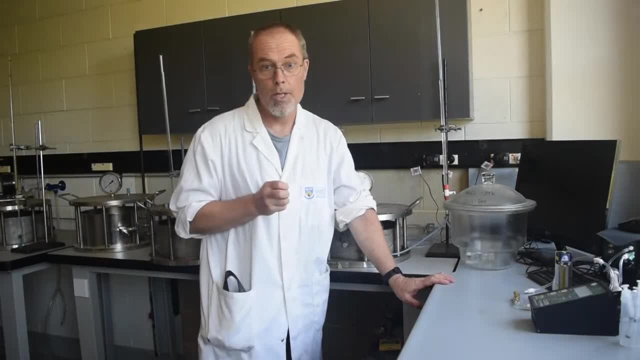 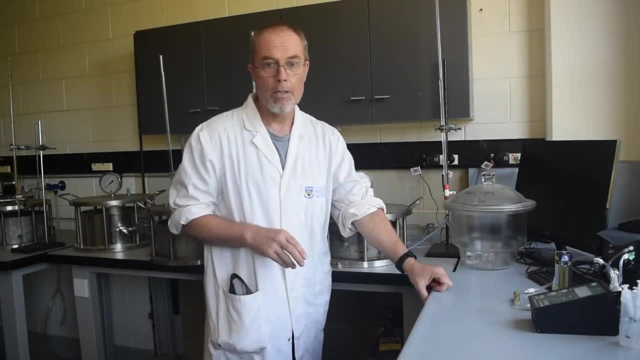 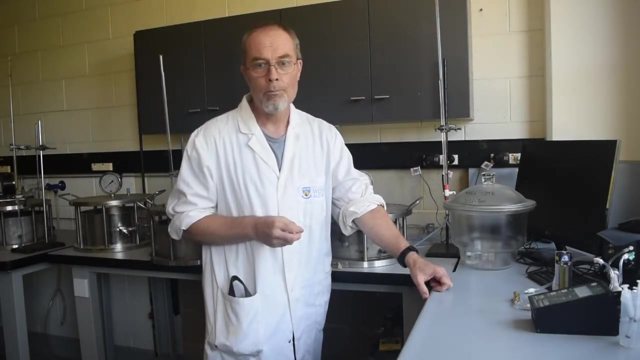 need to spend some time next week to measure the water content of the soil samples after they reach equilibrium at the various range of pressures that we use. and, of course, if you're putting wet samples in the oven, you need to come back at least a day later to measure the dry weight as well. Now, in terms of 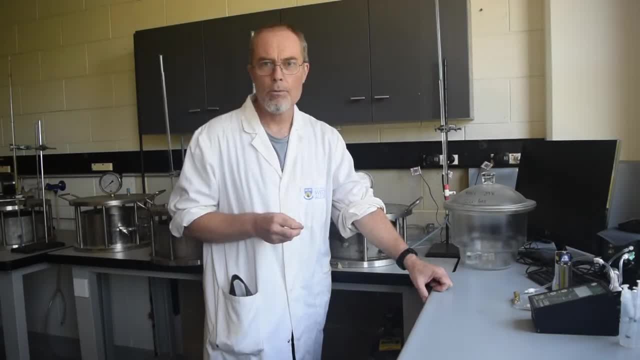 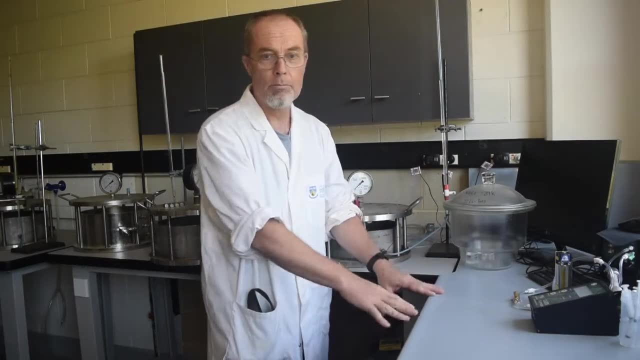 safety. there aren't really any serious safety issues for you. we do recommend that you wear latex gloves. You can get lab coats several times in the lab just because there may be residue on the benches which could do nasty things to your clothes and to keep yourself clean. but the more